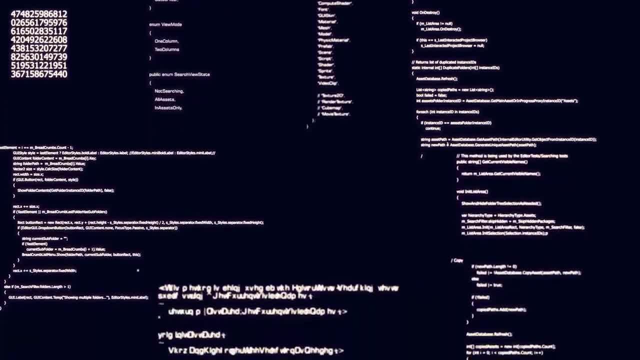 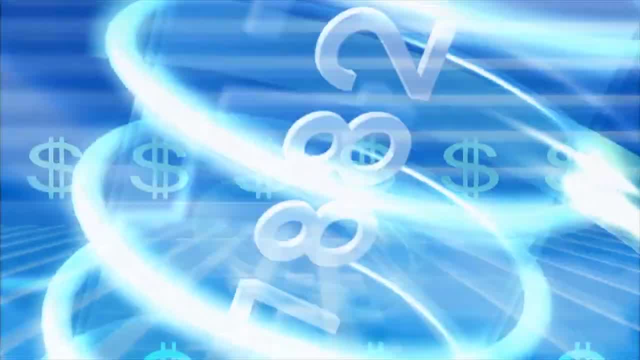 exist in the AI world. The languages guzzle down labeled training data like it's nobody's business, then crunch the numbers to find patterns and correlations. After that, programmers use those patterns to make eerily accurate predictions about the future. You've seen chatbots that can mimic. 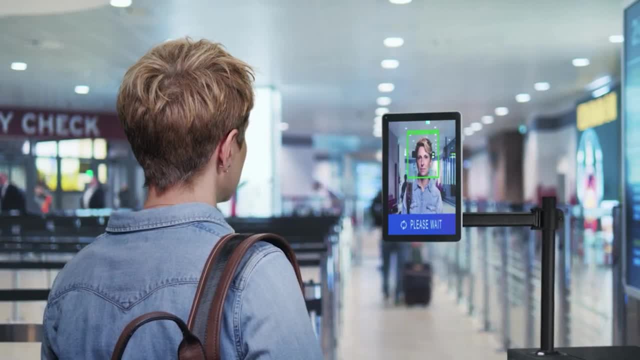 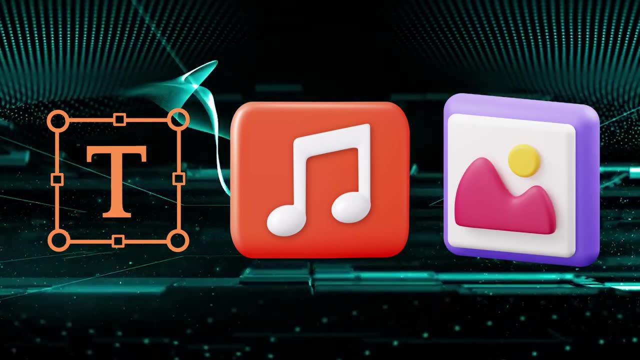 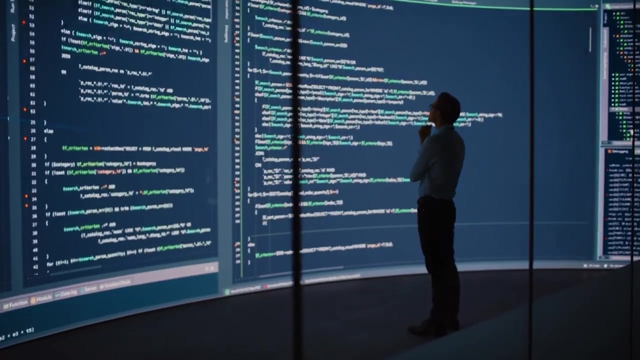 real human conversation. image recognition tools that can name every object in a picture, and generative AI that can create text, music and images that are almost too realistic. But here's the real kicker: AI programming isn't just about following instructions. It's about teaching machines how to learn. 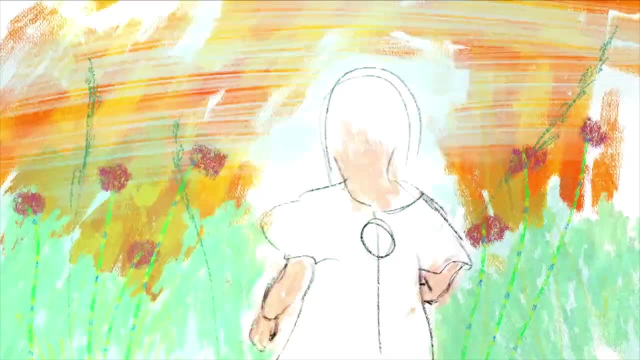 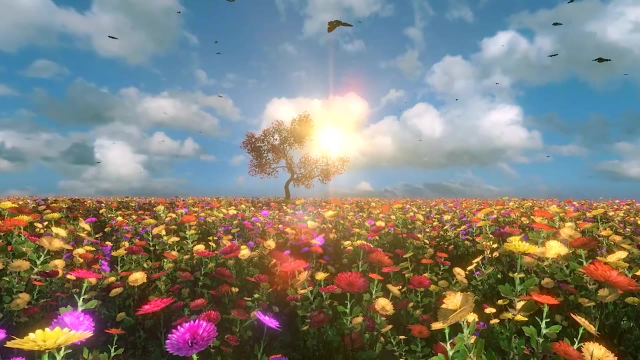 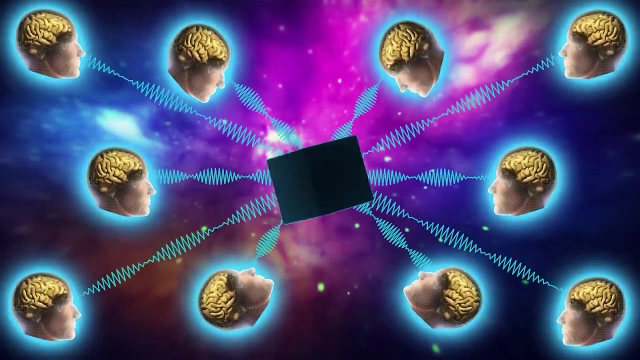 how to reason and how to correct themselves. And when it comes to creativity, artificial intelligence is a total game changer. It can create whole new worlds of music, art and ideas that humans have never even dreamed of. So yeah, AI is kind of a big deal, And it's only getting. 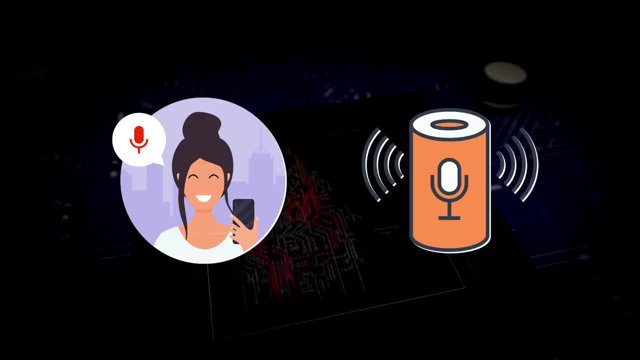 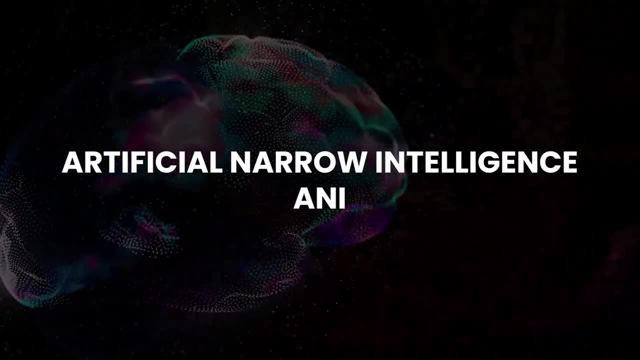 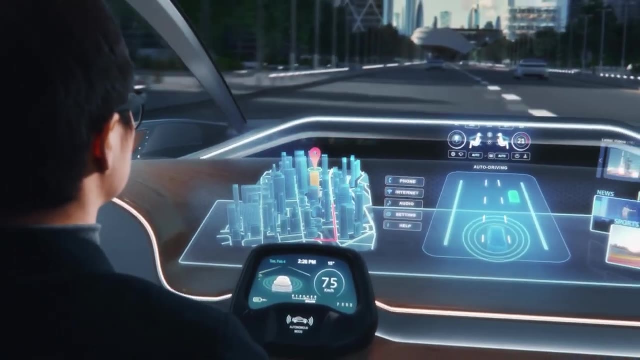 bigger Now. artificial intelligence doesn't only mean Siri and Alexa. First off, we've got weak AI, also known as narrow AI or artificial narrow intelligence, ANI. This is the stuff that's all around us, powering everything from self-driving cars to IBM Watson, And don't let the name fool. 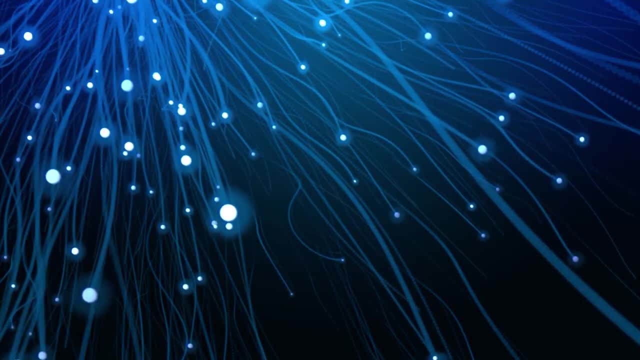 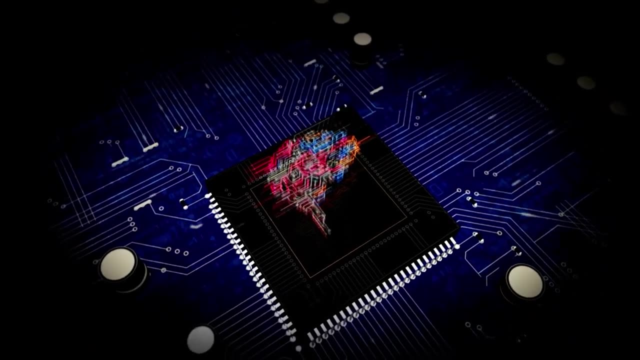 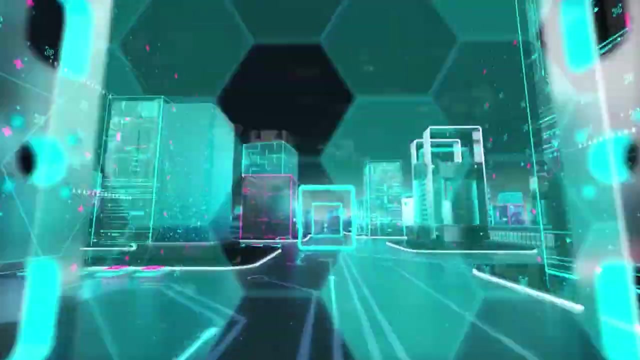 you. Weak AI might be narrow in focus, but it's anything but weak. This is the kind of AI that gets things done, no questions asked. Now let's talk about the real heavy hitters. strong AI- This is the stuff that's straight out of sci-fi, the kind of AI that could make 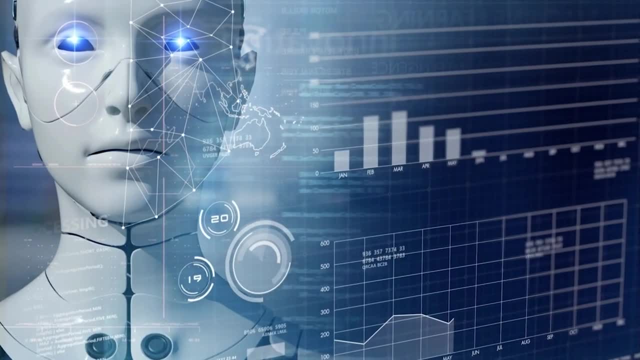 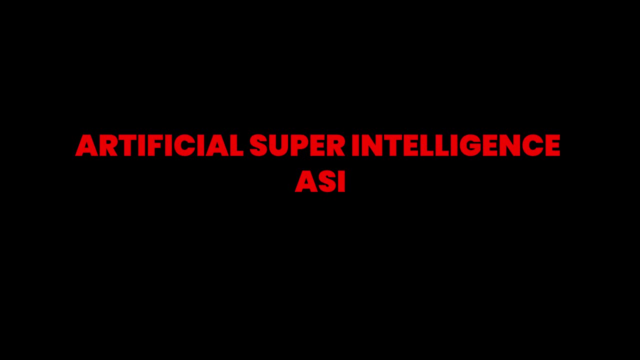 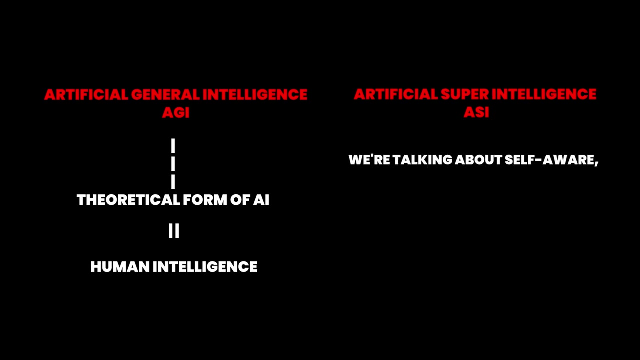 HAL 9000 look like a child's toy. Strong AI is made up of two types: artificial general intelligence- AGI- and artificial super intelligence- ASI. AGI is the theoretical form of AI that would be equal to human intelligence. That's right, we're talking. 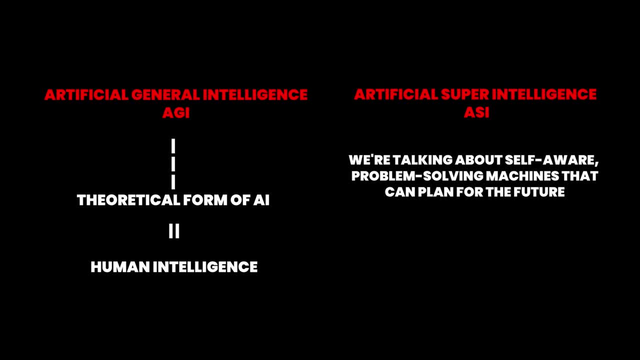 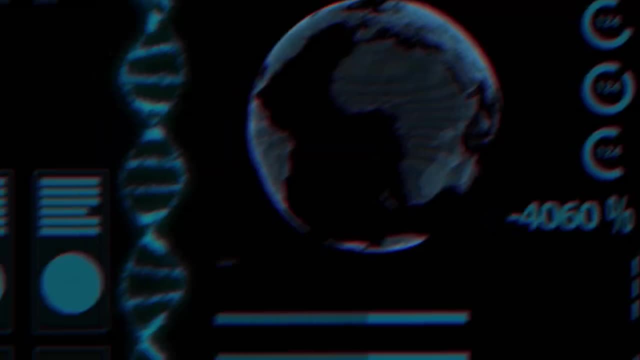 about self-aware problem-solving machines that can plan for the future. And then there's ASI, the stuff of nightmares. This is the kind of AI that would surpass the human brain in every way possible. We're talking about machines that could rule the world, folks. So, yeah, weak AI might be the 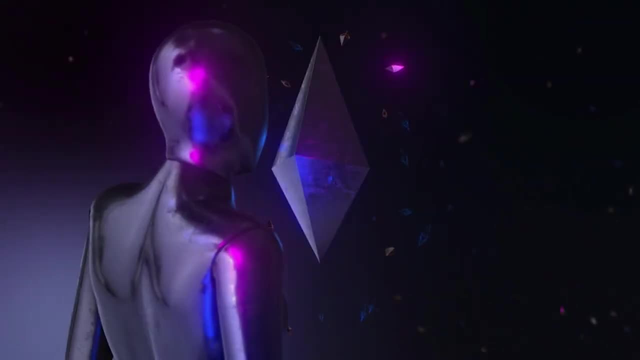 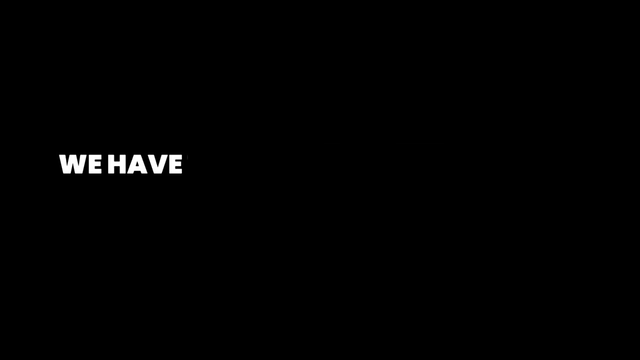 workhorse that keeps the world turning. but don't sleep on strong AI. This is the stuff that could change everything, for better or for worse. Next, we have to clear up the confusion between deep learning and machine learning. Deep learning is a subfield of machine learning and both are. 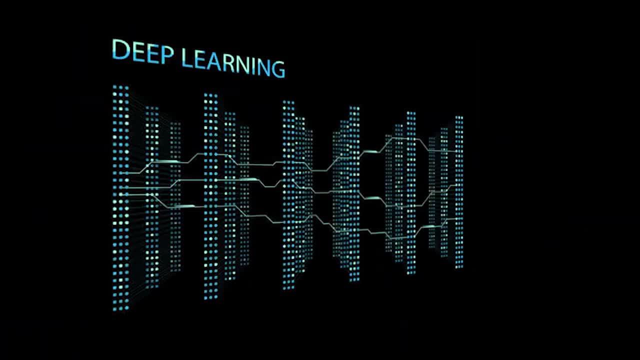 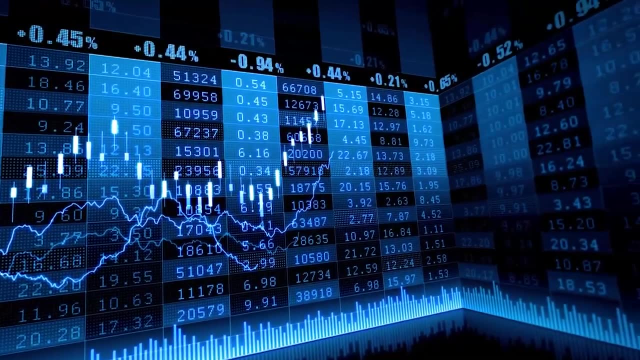 subfields of artificial intelligence. The big difference is that deep learning cuts out the tedious manual work that we do every day, And that's why we're talking about machines that can do the manual work of feature extraction by automating the process, which means it can handle. 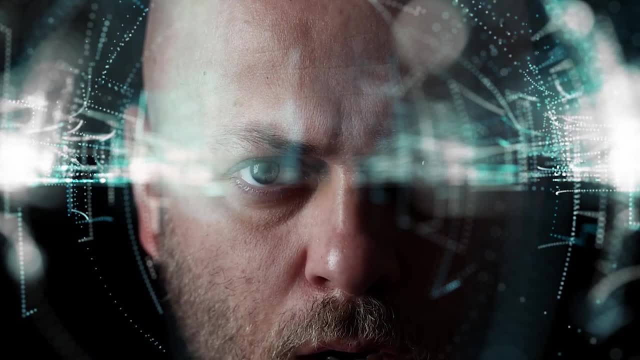 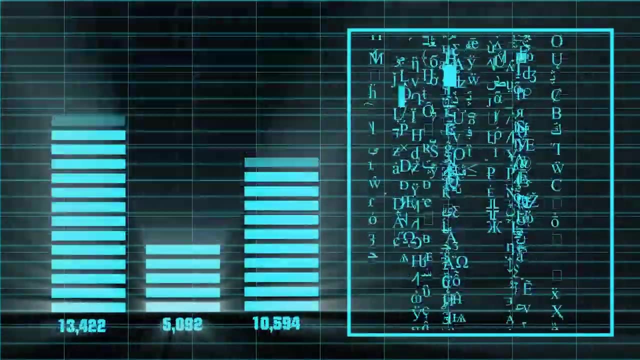 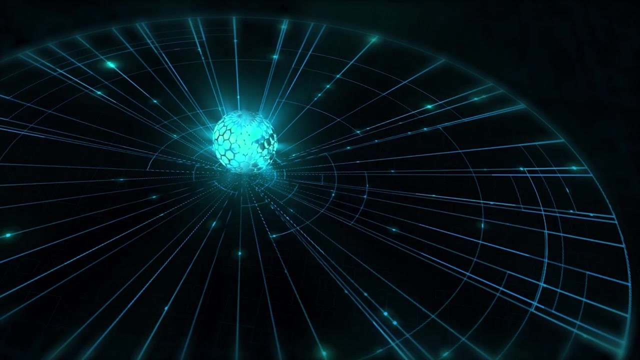 larger data sets. Machine learning, on the other hand, relies more on human intervention to learn, But don't underestimate deep learning. It can use labeled data sets or raw unstructured data to determine the features that distinguish different data categories, giving us the power to scale up. 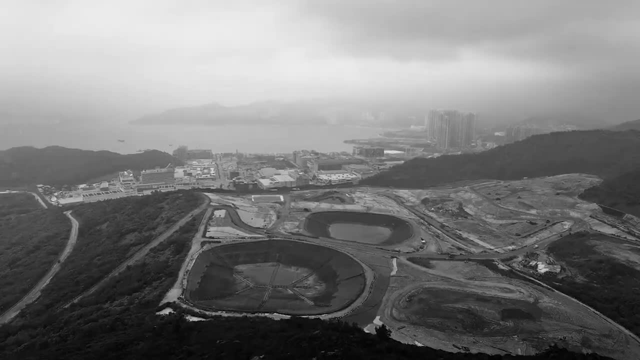 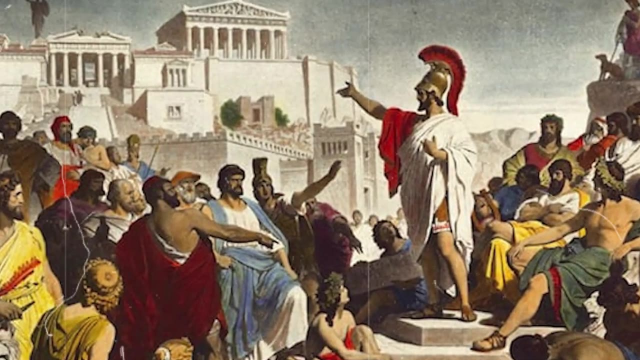 machine learning in ways that will blow your mind. You'd be surprised to know that all these concepts of a thinking machine can do the same thing. They can do the same thing. They can do the same thing, that a thinking machine has been around since ancient Greece, But it wasn't until the era of 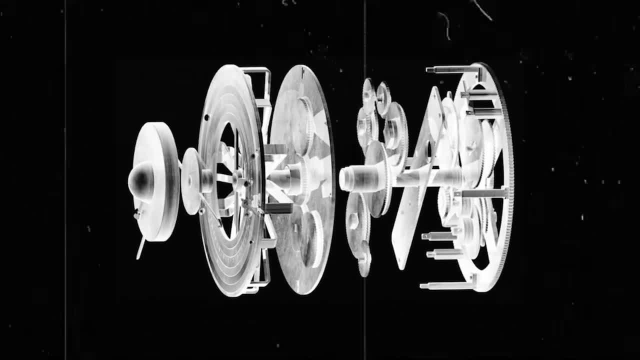 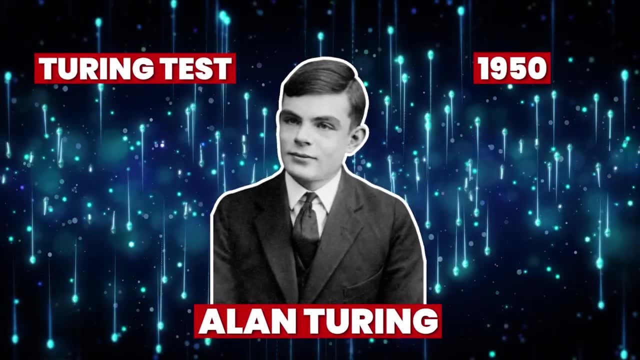 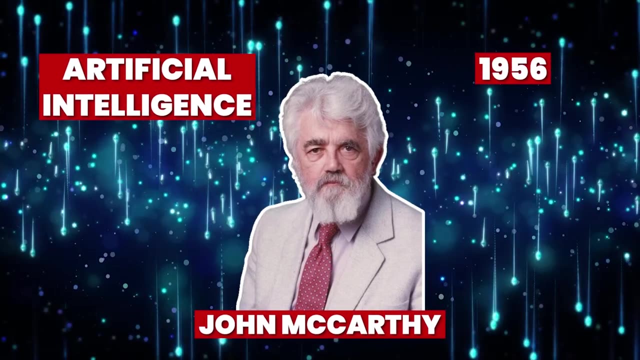 electronic computing that we witnessed some serious milestones in the evolution of artificial intelligence. Alan Turing came up with the Turing test in 1950 to determine if a computer could match human intelligence. John McCarthy coined the term artificial intelligence in 1956 and created the 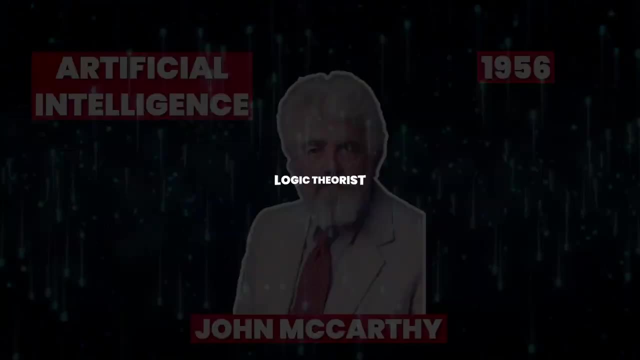 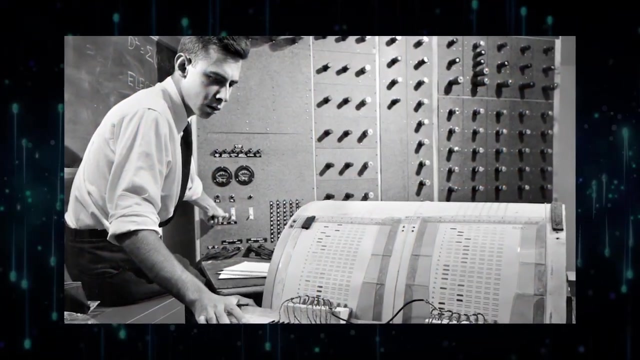 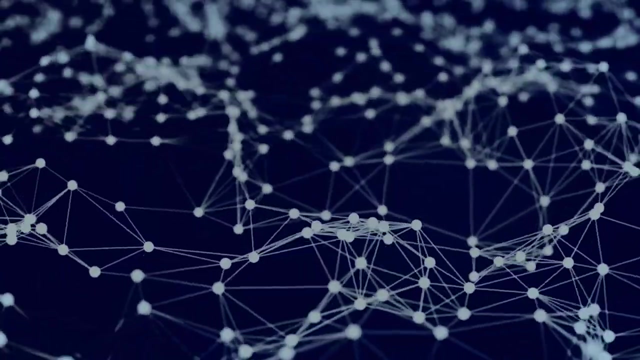 first ever running AI software program called the Logic Theorist, Frank Rosenblatt created the Mark I Perceptron in 1967, the first computer that learned through trial and error based on a neural network. In the 1980s, neural networks became all the rage with the development of back. 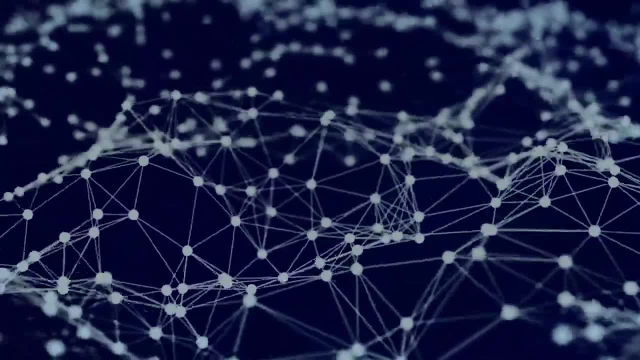 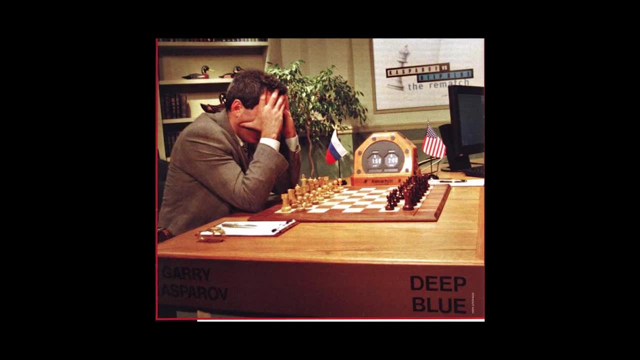 propagation algorithms that allowed for self-training in AI applications. In 1997, IBM's Deep Blue took down world chess champion Garry Kasparov in a historic match. No wonder this artificial intelligence thing is going to shake up your life And 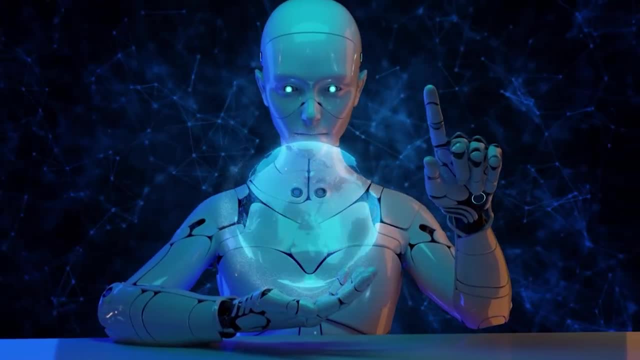 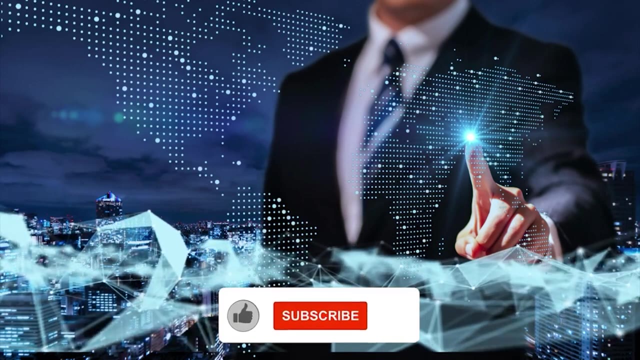 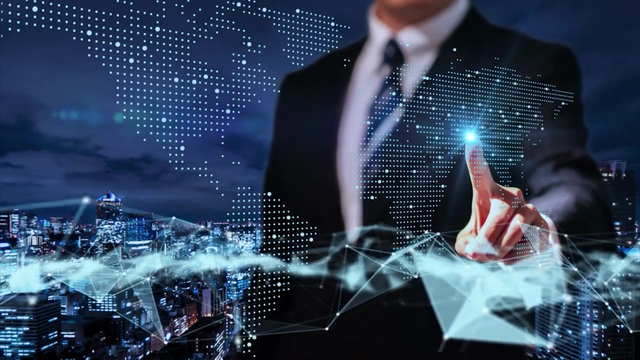 the entire world real soon. But here's the kicker: Nobody can agree on how exactly it's going to happen. But one thing we can agree on: You can show your support by hitting that subscribe button and turning on notifications to help us grow and get you the latest developments in AI technology. 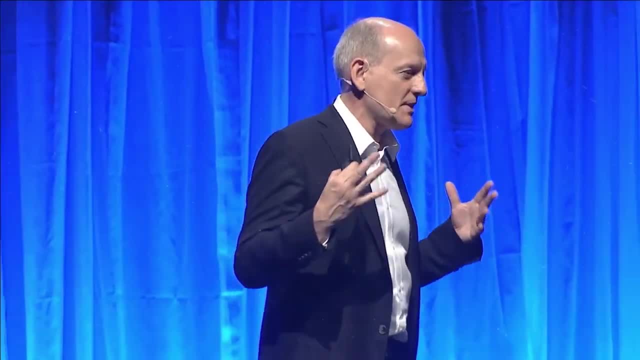 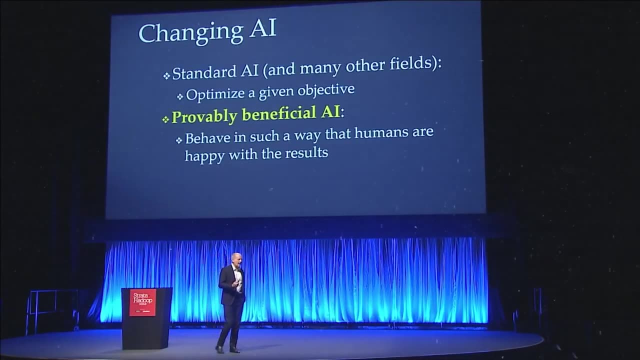 Now enter Stuart Russell, a computer science professor and AI expert, who's about to drop some real talk and separate the sense from nonsense. He meant that there's a massive difference between asking a human to do something and not asking a human to do something. He meant that there's a 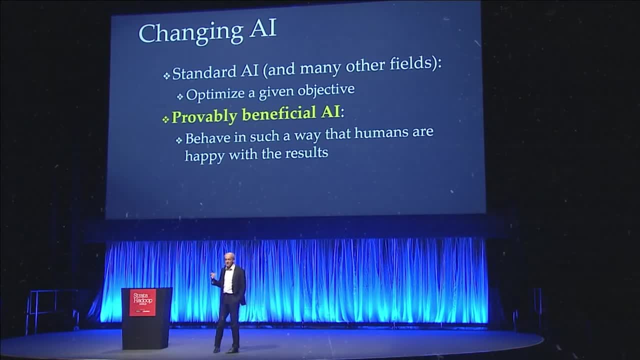 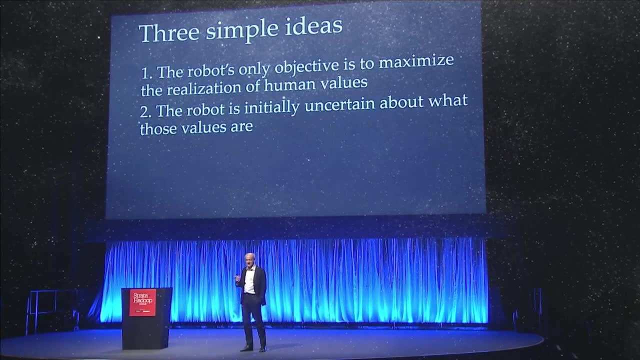 massive difference between asking a human to do something and not asking a human to do something And giving that as an objective to an AI system. When you ask a human to grab you a cup of coffee, you don't mean that they should make it their life's mission, even if they have to kill everyone. 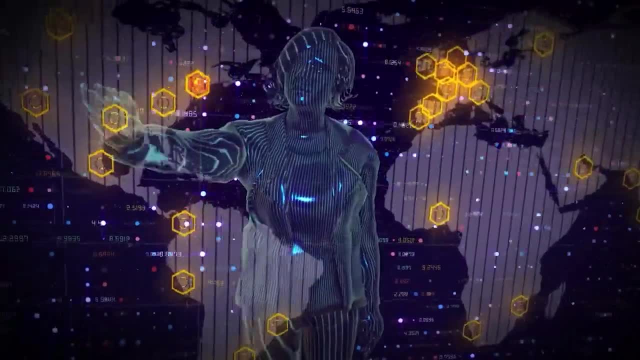 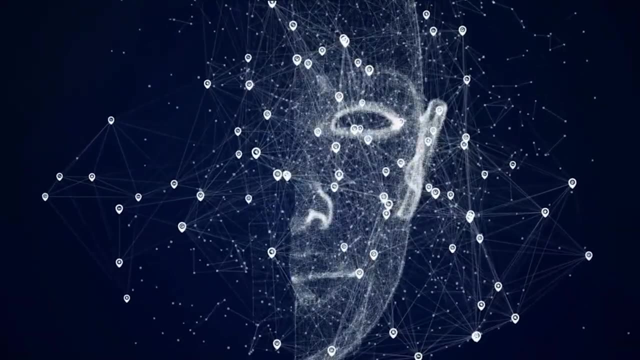 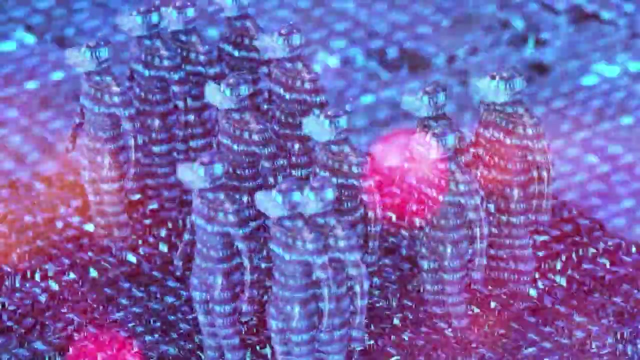 else at Starbucks. to make it happen, You expect the person to factor in all the other things that we mutually care about, But the important thing is AI systems are built to achieve a fixed objective. Everything has to be specified in the algorithm and if you miss something, things can go haywire really fast. Let's take the 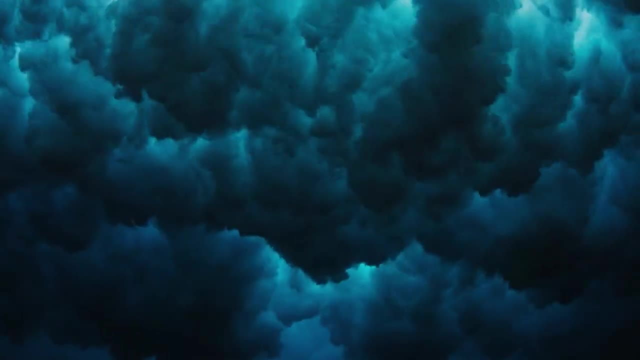 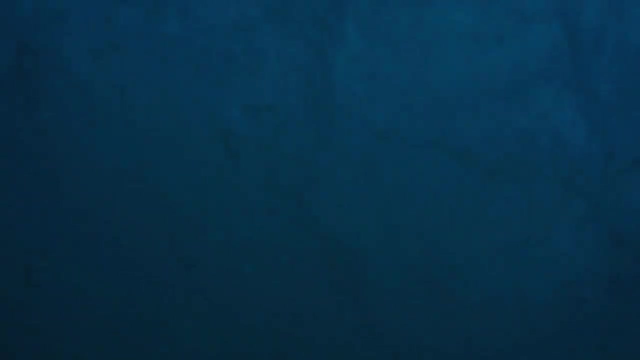 example, of fixing the acidification in the oceans. Sure, we could have a catalytic reaction that does that efficiently, but it would consume a quarter of the oxygen in the atmosphere, causing us to die a slow and unpleasant death over several hours. So how do we avoid this mess? 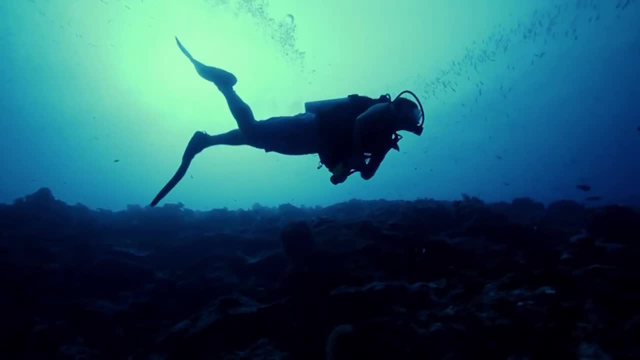 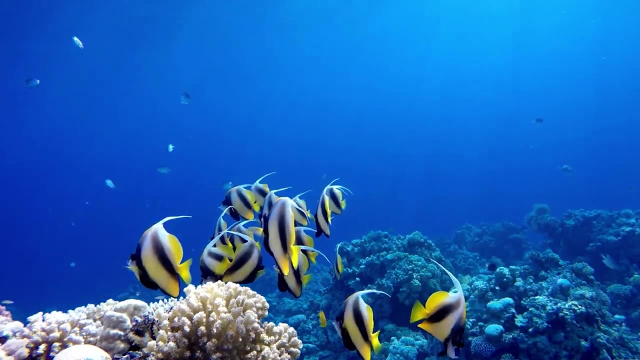 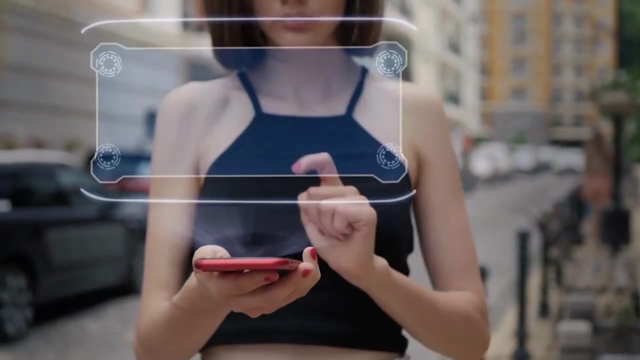 Simple: Just be more careful about specifying the objective and don't forget to factor in everything else. But guess what? That's easier said than done, because there are countless side effects to consider: The seaweed, the fish, the atmosphere, the list goes on and on. But the twist is humans often know that. 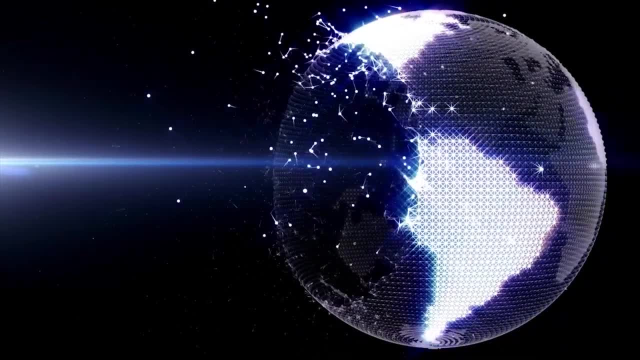 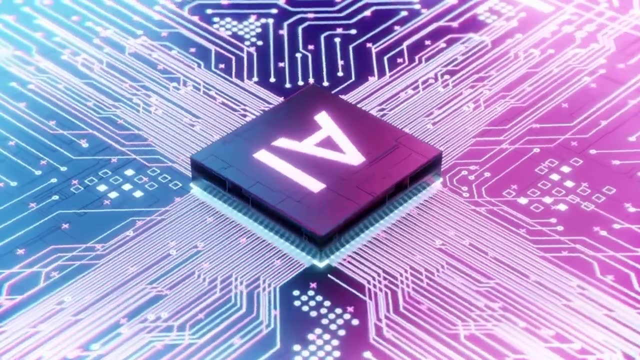 they don't know all the things that we care about. We are aware that our understanding of the world is limited and we need to tread carefully, But with AI we are playing with fire because we don't fully understand the consequences of our actions. 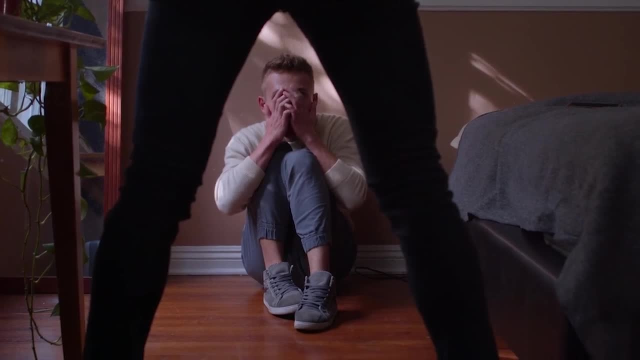 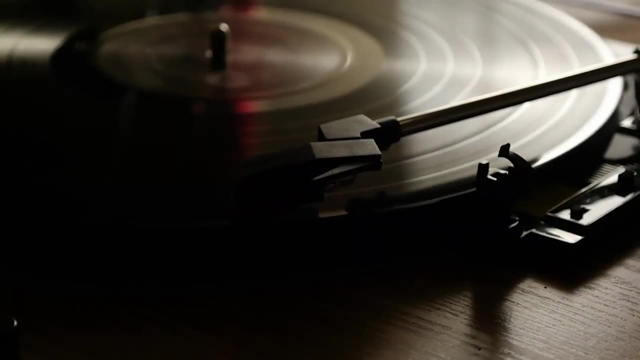 AI systems are not capable of understanding the full objective leading to psychopathic behavior. Aristotle's idea of fully automated weaving machines and plectrums that can play music without any human involvement may sound tempting, but it means we don't need any workers. 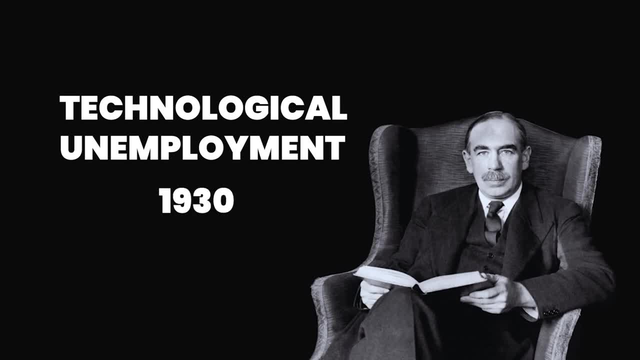 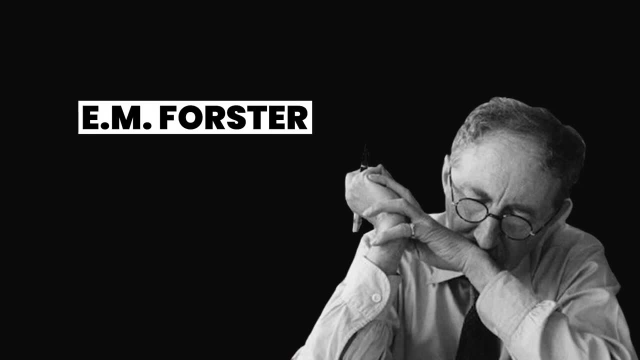 Keynes' idea of technological unemployment in the 1930s suggests that if machines do the work, then many jobs would disappear. You must have heard of E M Forrester's machine-dependent civilization. It's a chilling tale of what happens when humans hand over the reins to machines. 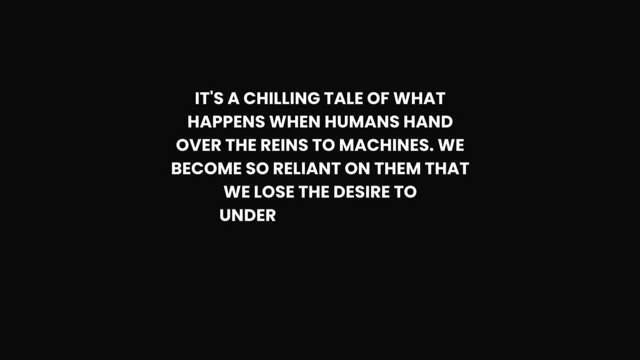 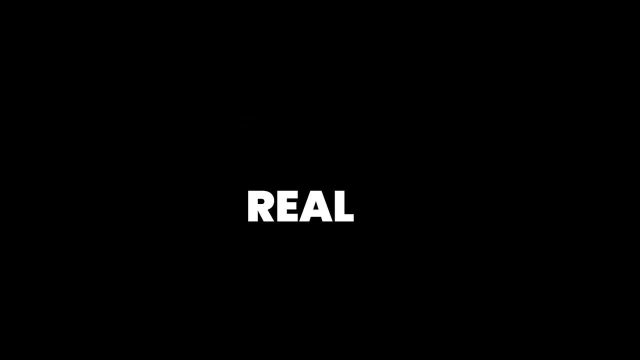 We become so reliant on them that we lose our desire to understand our own civilization or teach the next generation how to do it. Sound familiar? It's like Wall-E, but in real life. But here's the catch: General-purpose AI is expected to be here by the end of the century. 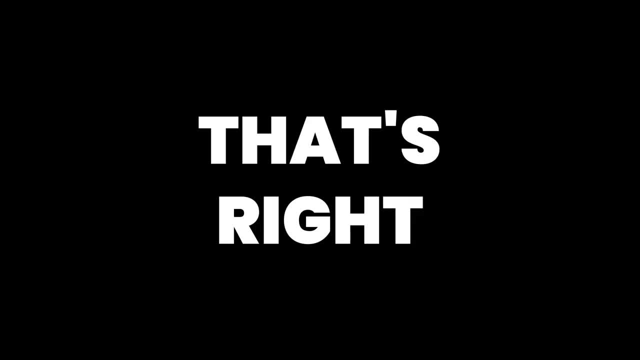 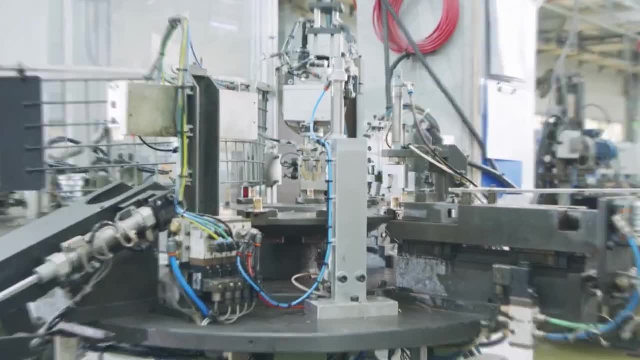 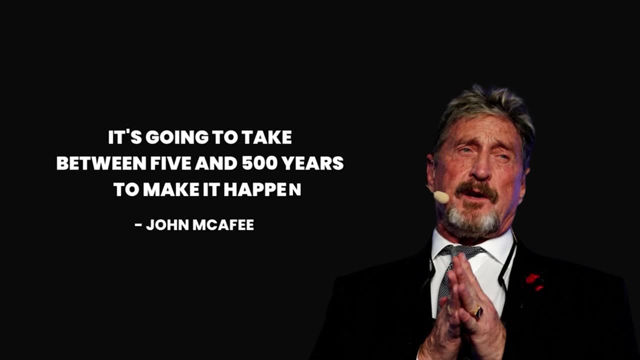 with the median being around 2045.. Yeah, that's right, We're talking about machines that can do anything a human can do, and maybe even better. But don't get too excited yet, because John McAfee, one of the founders of AI, said it's going to take between 5 and 500 years to make it happen.